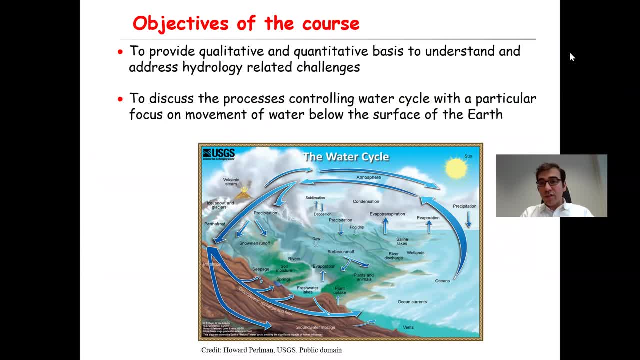 basis to understand and address hydrology related challenges, as well as to discuss the processes controlling water cycle, with a particular focus on movement of water below the surface of the earth. Okay, so these are the two main objectives of this course In terms of the textbooks I use. 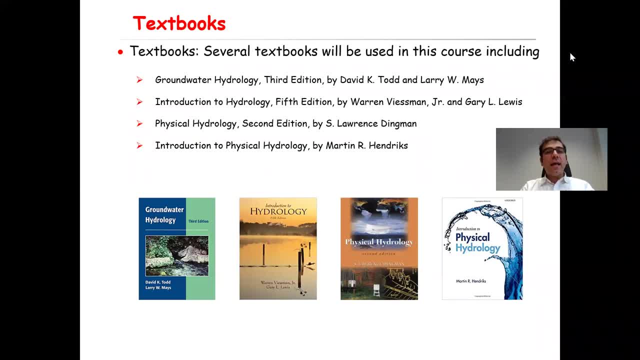 several books to prepare these lectures, but the main four textbooks that I use are listed below. that is, groundwater hydrology by Todd and Mays, introduction to hydrology, physical hydrology and introduction to physical hydrology. Okay, in terms of the syllabus. so the first chapter is: 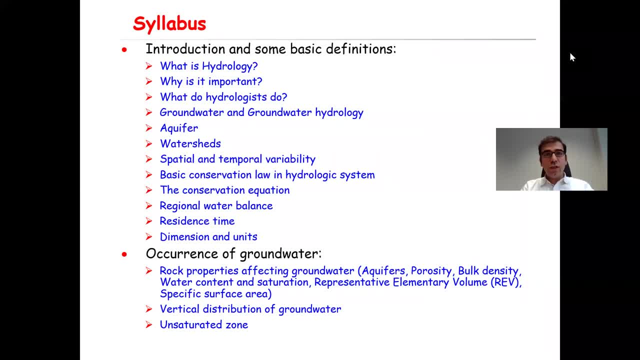 introduction and some basic definitions, which I hope to cover in this lecture, where we will discuss about what is hydrology, why is it important? what do hydrologists do? groundwater and groundwater hydrology. We will provide the definition of aquifer watersheds and also a few. 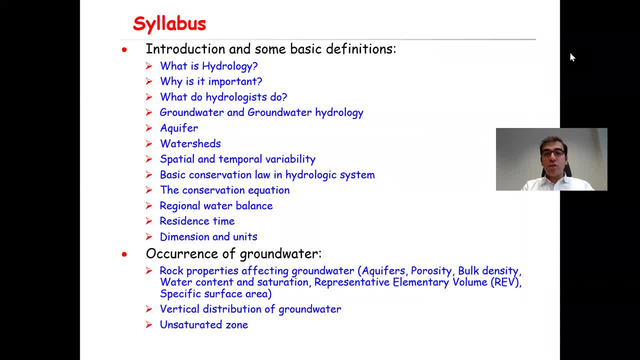 words on a special and temporal variability. We talk about the basic conservation law in hydrologic systems. We talk about the conservation equation, the regional water balance, residence time and the differences between units and dimensions. That is chapter one. Okay, and the next chapter will be. 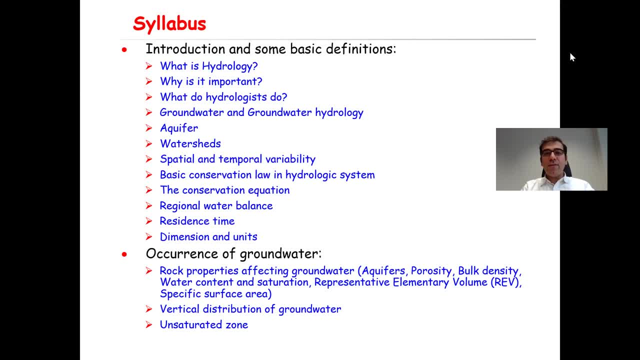 about occurrence of groundwater, where we talk about rock properties affecting groundwater, that is, the type of aquifers, porosity, rock density, water continent saturation, representative elementary volume, the concept of REV, basically, and a specific surface area. Then we talk about 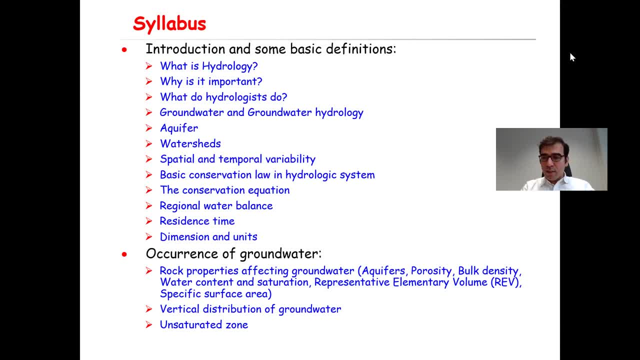 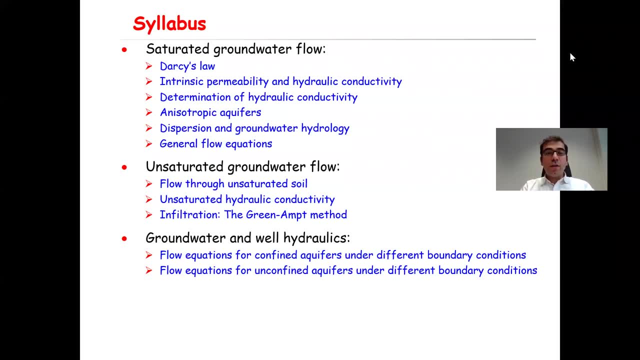 vertical distribution of groundwater and we talk about unsaturated zone. That chapter will be followed by a new chapter on saturated groundwater flow, where we talk about Darcy's law, we talk about intrinsic permeability and hydraulic conductivity. we talk about determination of hydraulic conductivity, anisotropic aquifers, dispersion and groundwater. 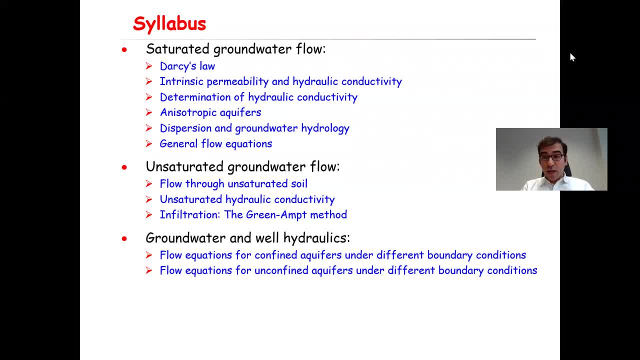 hydrology, as well as general flow equations. Okay, and then the next chapter will be about unsaturated groundwater flow, which is about where we will talk about flow through unsaturated soil, unsaturated hydraulic conductivity and the process of infiltration, and we will talk 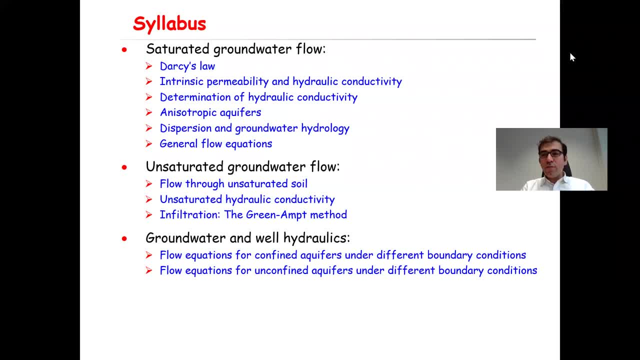 about the Green App method. Okay, and then the last chapter of this course will be about groundwater and well hydraulics, where we talk about flow equations for confined aquifers under different boundary conditions, as well as flow equations for unconfined aquifers under different boundary. 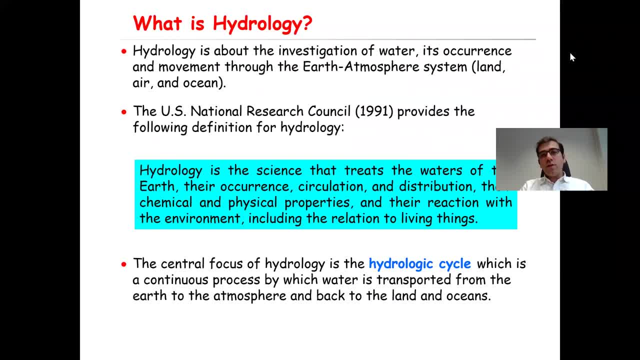 conditions. Okay, so what is hydrology? Hydrology is basically the science of the investigation of water movement in earth and atmosphere system. In other words, hydrology is about the investigation of water, its occurrence and movement through the earth's atmosphere system, and by that I mean land. 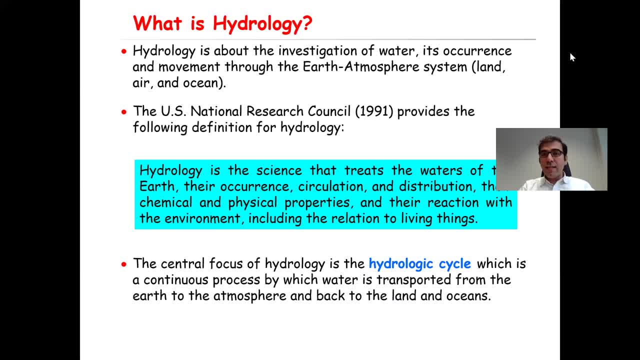 air and ocean. The USNRC, or National Research Council, provides the following definition for hydrology: That is: hydrology is the science that treats the waters of the earth, their occurrence, circulation and distribution, their chemical and physical properties. 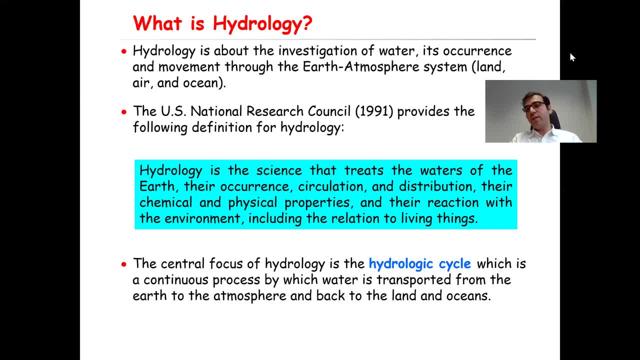 and their reaction with the environment, including the relation to living things. Okay, so that is the official definition of hydrology by USNRC. Okay, the central focus, the central focus of hydrology, is the hydrologic cycle, okay, which is a continuous process. 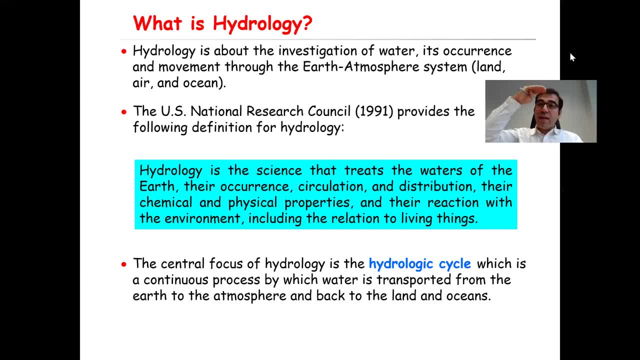 by which water is transported from land to the atmosphere and again back to the back, from atmosphere to the land and ocean. So analysis of the hydrologic cycle is basically the central focus of the hydrologic sciences, And so hydrologic science- sorry, hydrologic cycle- is usually 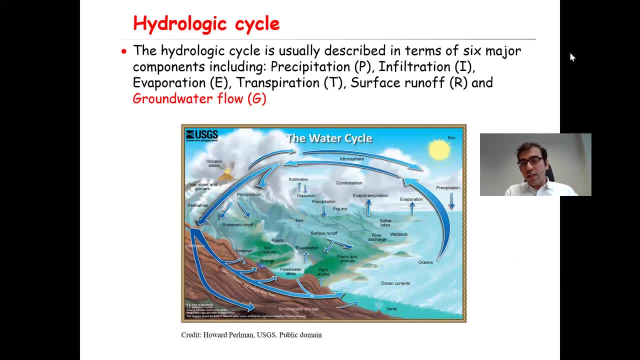 described in terms of six major components, including precipitation, presented by P, infiltration I, evaporation- E. transpiration, presented by T, that is because of the vegetation and plants and so on, surface runoff and groundwater flow, which is presented by G. 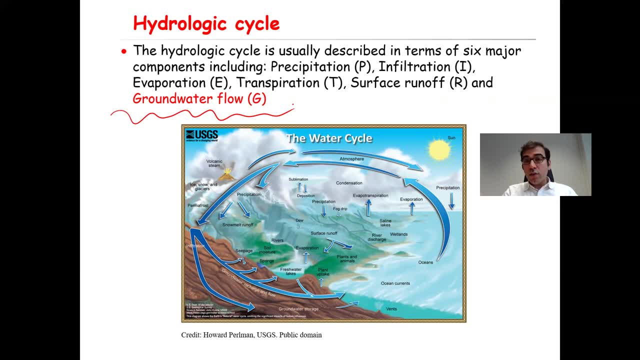 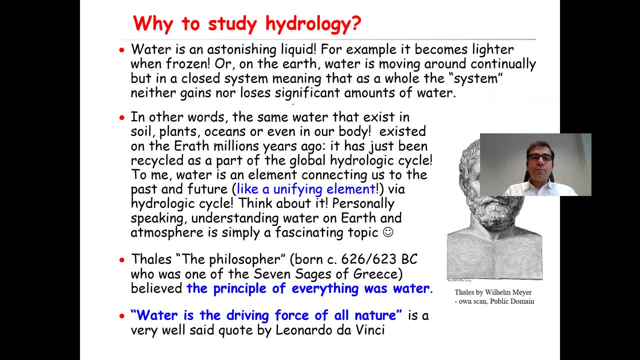 and that is the focus of this course. okay, So these are the major components of the hydrologic cycle. okay, So why to study hydrology? I was not sure to present this slide or not. This is like my own personal view. 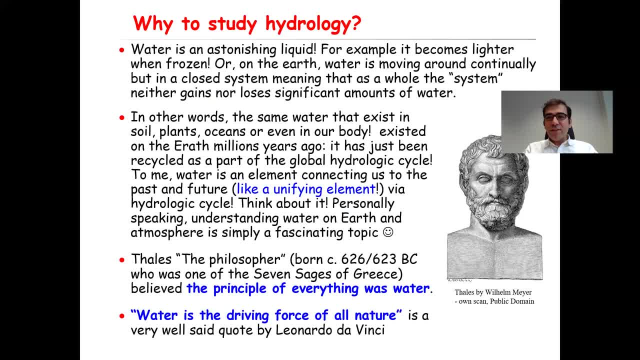 but I thought it would not harm to explain that, And after that I will explain more. let's call it like a scientific, more scientific reason actually why we need to study or to have a clear understanding about hydrology. To me, from like personally speaking, I find water as a kind. 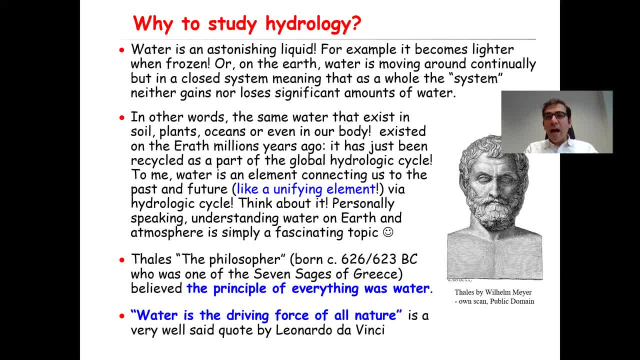 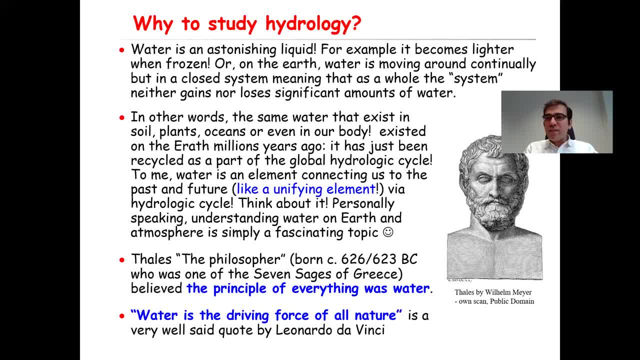 it freezes, it is lighter. That is like a very interesting concept. right Or on the earth, water is moving around continually, but in a closed system. What does it mean? It means the system as a whole neither gains nor loses a significant amount of water, In other words, the 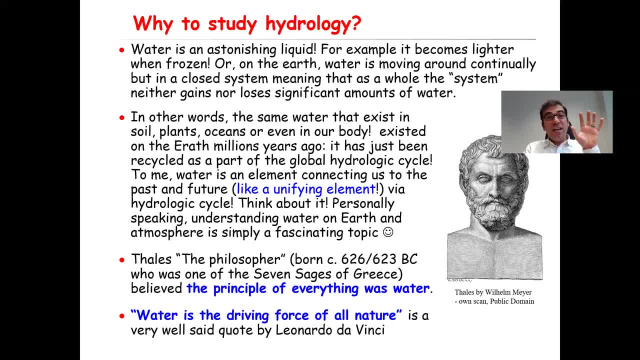 same water that exists, let's say, in soil, in plants, in ocean or even in our body. the same water actually exists in our body. So it's the same water that exists, let's say, in soil, in disorder cream or even أن ج mil fique'یου es. 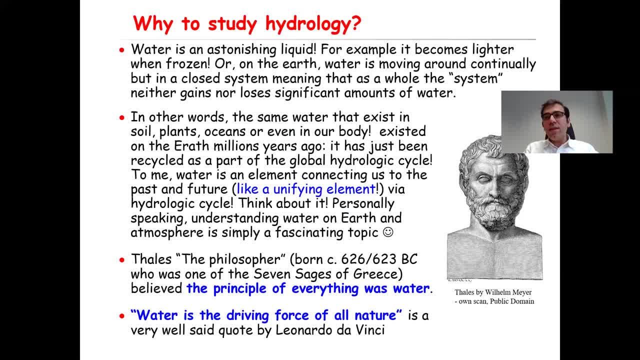 way. So it's the same water that exists. it is the same water that exists for democracies and so on too, Like what it says in textbooks. And second is that water has existed since millions of years ago on earth and it has just been recycled through the hydrologic. 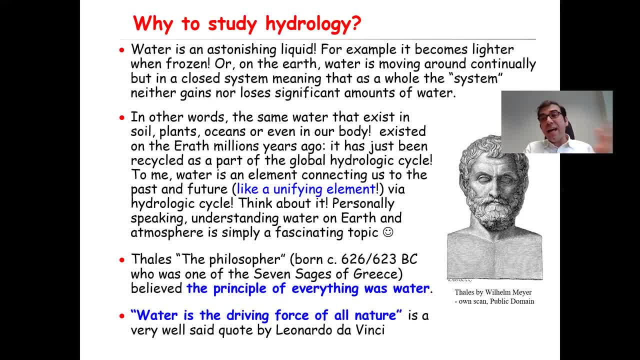 cycle. So to me, water is a kind of an element that is connecting us to the past and to the future like a unifying element via hydrologic cycle. So think about it. this is like a very interesting concept That, personally speaking, understanding water on earth and atmosphere is. 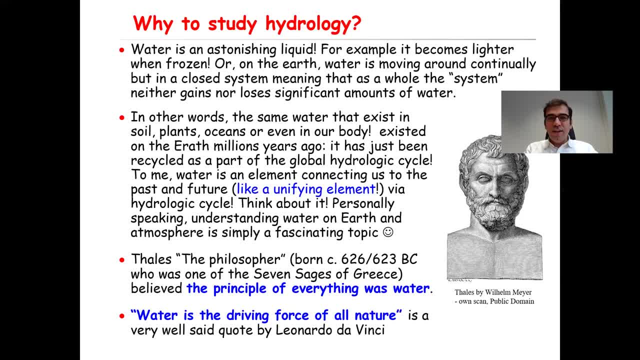 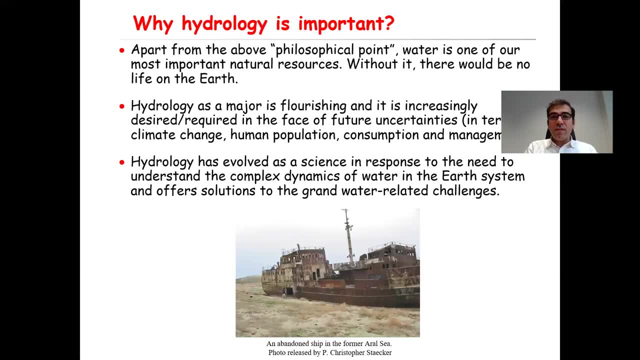 OK, so tell us, the great Greek philosopher believed the principle of everything was water, and water is the driving force of all nature. This is a very well said quote by Leonardo da Vinci. OK, so, but of course, above this philosophical point, if you want to call it, water is one of our most important natural resources and assets. 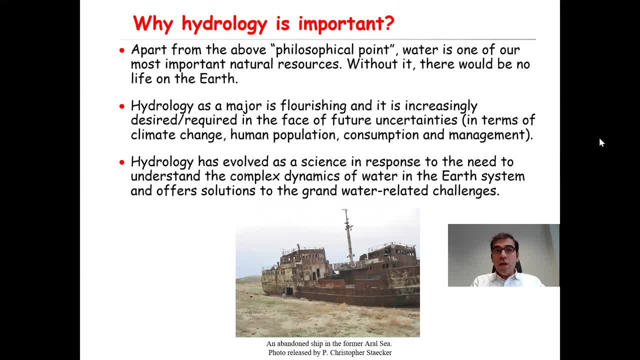 Without it, as you know, there would be no life on the earth, Right? So hydrology as a measure is flourishing and it is increasingly desired, required in the face of future uncertainties, And when I say uncertainties, I mean in terms of climate change, in terms of human population, in terms of water consumptions and in terms of management. 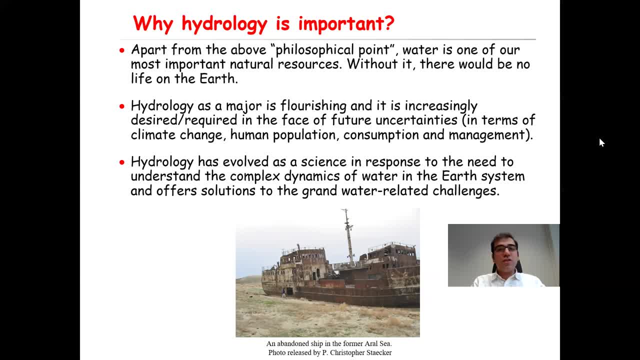 OK, so that is more and more it is needed to understand, to have a clear understanding about hydrology, And hydrology has evolved as a science in response to the need To understand the complex dynamics of water in the air system and offer solutions to the grand water related challenges. 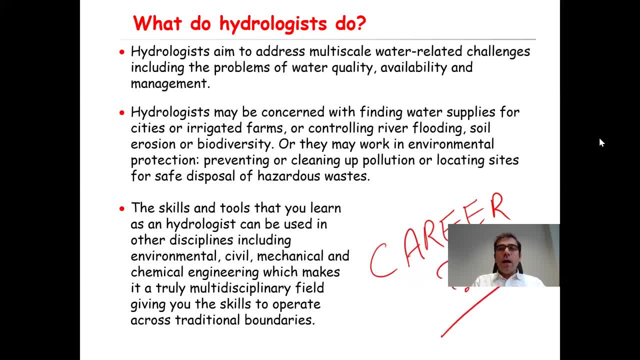 OK, so what do hydrologists do? Hydrologists aim to address multiscale water related challenges, And when I say multiscales, by definition hydrology is a multiscale science. For example, the problems they investigate sometimes ranges from nanoscale or microscale up to the global scale. 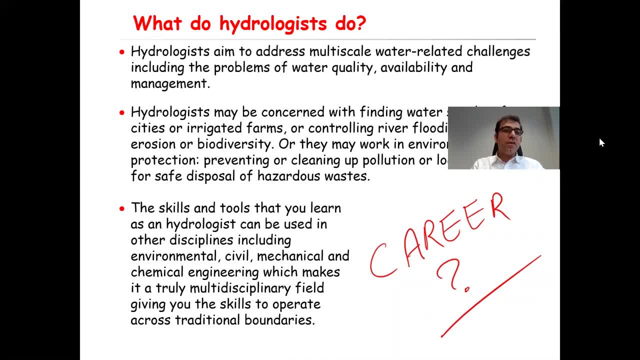 So, by definition, It's a multiscale science. So hydrologists aim to address multiscale water related challenges, including the problems of water quality, availability and management. OK, so hydrologists may be concerned with finding water supplies for cities or irrigated farms, or controlling river flooding, soil erosion or biodiversity. 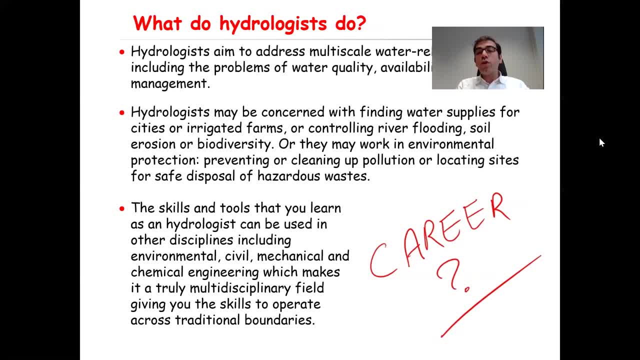 Or they may work in environmental protection, preventing or cleaning up pollution or locating sites for safe disposal of hazardous waste. So this is another type of work the hydrologists do. But in my opinion, the skills and tools that you learn as a hydrologist, you can apply those tools and skills and knowledge. 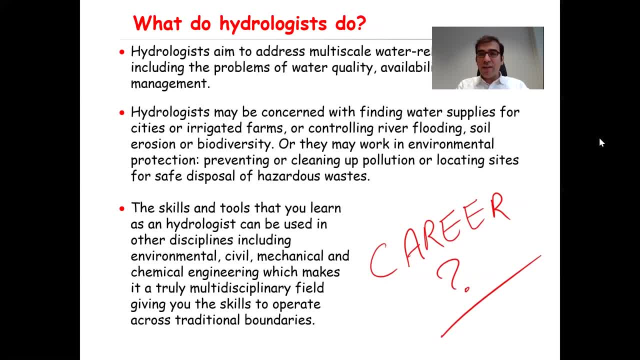 in different disciplines, For example, environmental engineering, definitely civil engineering, chemical engineering, mechanical engineering. In all these sciences you can use and apply the tools you learn as a hydrologist. Therefore, it is, by definition, is a multidisciplinary field which gives you the opportunity to operate basically. 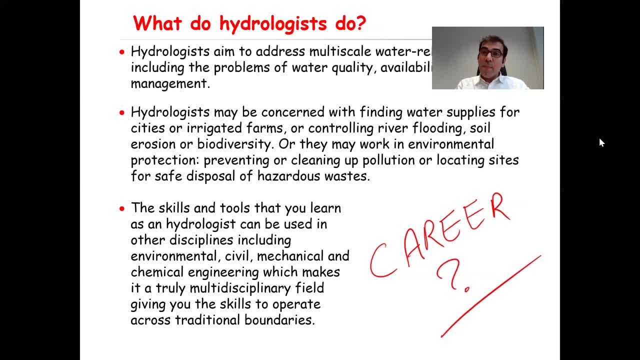 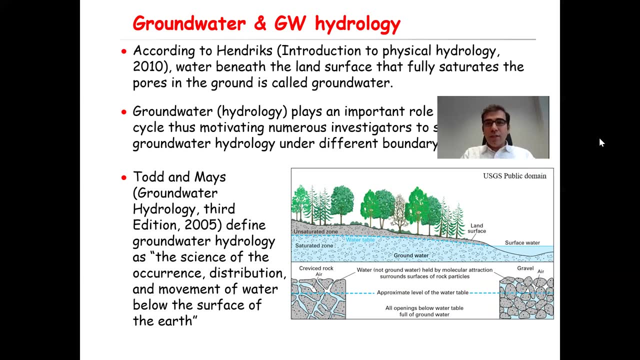 across traditional boundaries And that will basically provide you with a better job opportunity. Okay, so that is what hydrologists do. So groundwater and groundwater hydrology, According to Henrik's introduction to physical hydrology, which is one of the textbooks that 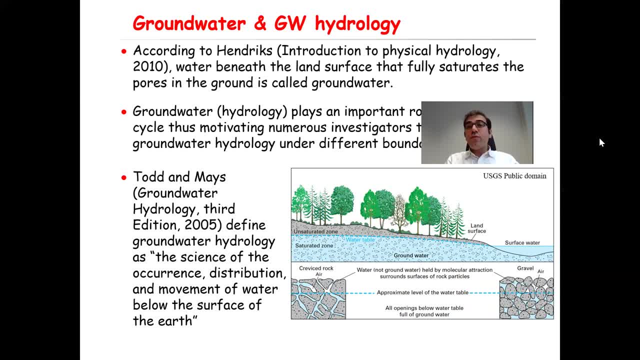 he used in this paper. he said you can use the tools you learn as a hydrologist, and we also can use the technologies to design or mean, so that you can tell of um intentions or values as well, And this is also related to the physical humanities, and they're all kannst of. 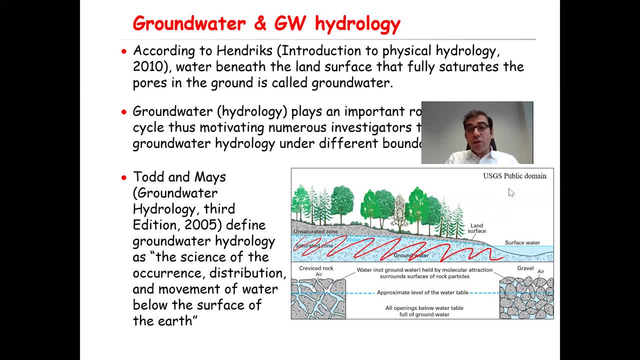 the experience very similar. So people's Alaska skills right. So if you are keen toself learn for yourself in this domain, you take the CT scan. so this tissue looks at important points, holds some technique that you will need when you you know you think about, for example, 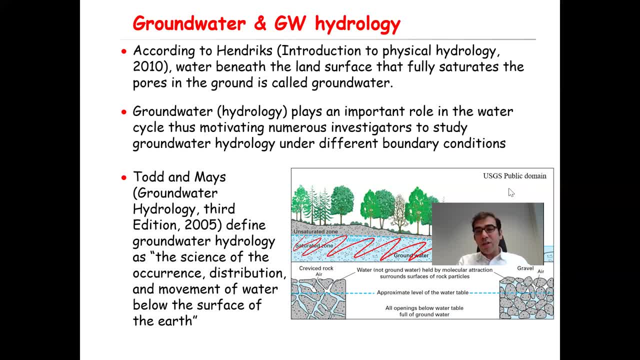 Therefore, it is important to have a clear understanding about groundwater hydrology, to be able to describe the water cycle, And this very fact motivated many investigators to study groundwater hydrology on the different boundary conditions. OK, so Todd and May's Groundwater Hydrology, which is another textbook that I use in this lecture. 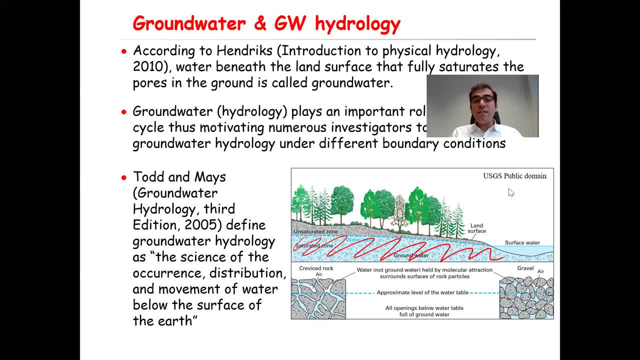 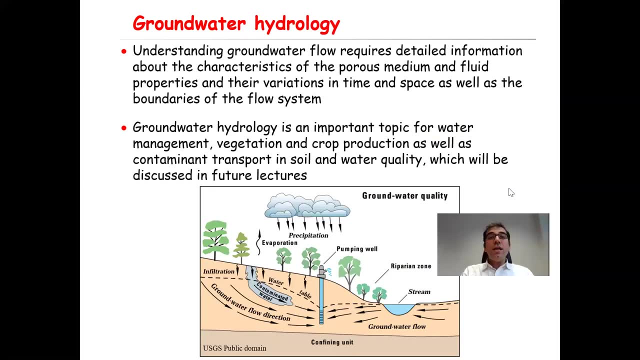 defined groundwater hydrology as the science of the occurrence, distribution and movement of water below the surface of the Earth. OK, so that is the definition of groundwater hydrology given by Todd and May's. OK, so groundwater hydrology: understanding groundwater flow requires detailed information about the characteristics of the porous medium. 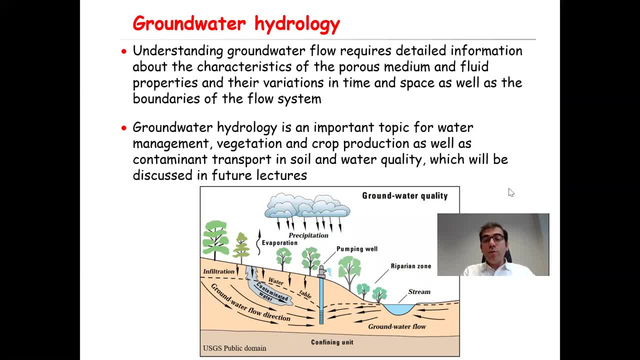 means soil, underground reservoirs, rocks, etc. and fluid properties and their variations in time and space, as well as the boundaries of the flow system. Groundwater hydrology is an important topic for water management, vegetation and crop production, as well as contaminant transport in soil and water quality, which will be discussed in future lecture. 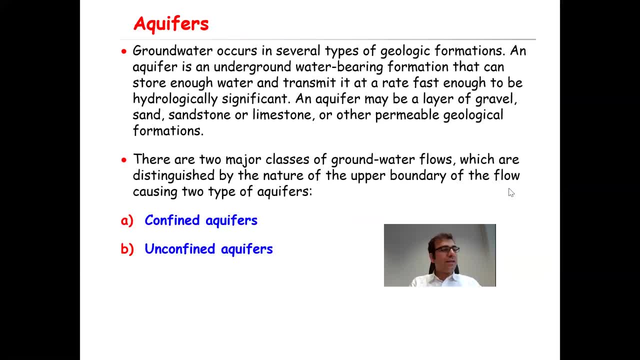 OK, so aquifer, what is aquifer? Aquifer is actually. you hear the word aquifer quite often in hydrologic terminology, in hydrologic textbook. And what is aquifer? So, as mentioned already, groundwater occurs. It's in several types of geologic formation. 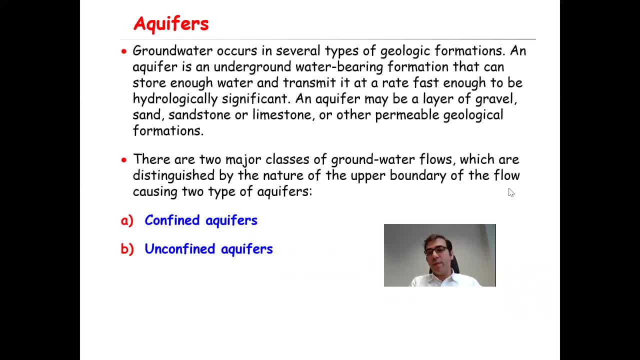 An aquifer is an underground water-bearing formation, OK, that can store enough water and, at the same time, that can transmit it at a rate fast enough to be hydrologically significant. So that is an aquifer. So, as you can imagine, aquifer can be, or may be, a layer of gravel, sand, sandstone, limestone or other or any other permeable geological formation. 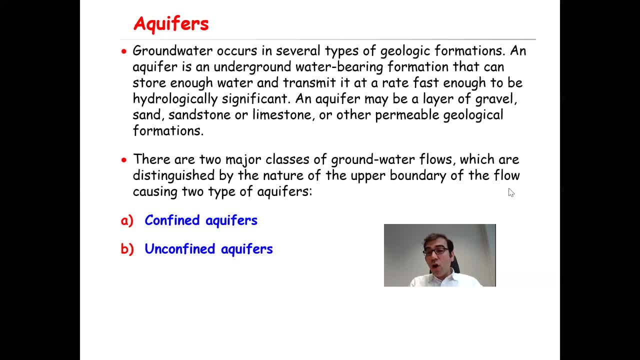 OK, so depending Depending on the upper boundary of the aquifer, you have two main types of aquifer, That is, confined and unconfined aquifer. So there are two major classes of groundwater flows which are distinguished by the nature of the upper boundary of the flow. 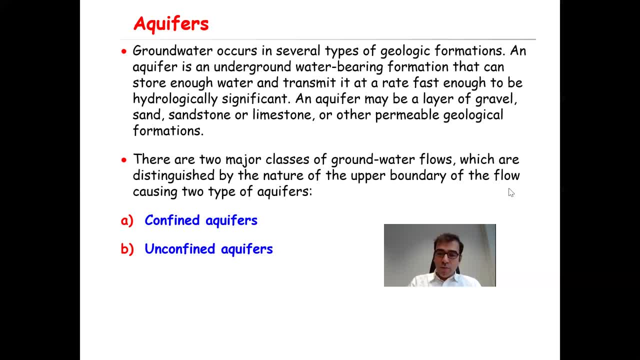 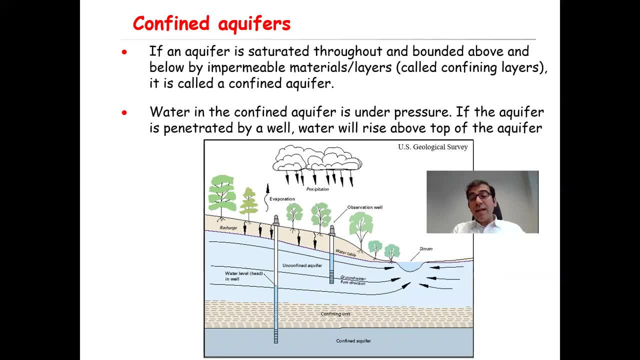 causing two types of aquifer: confined aquifers and unconfined aquifers. OK, so what is confined aquifer? Confined aquifer is a confined aquifer. If an aquifer is saturated, completely, fully saturated, it's a confined aquifer. 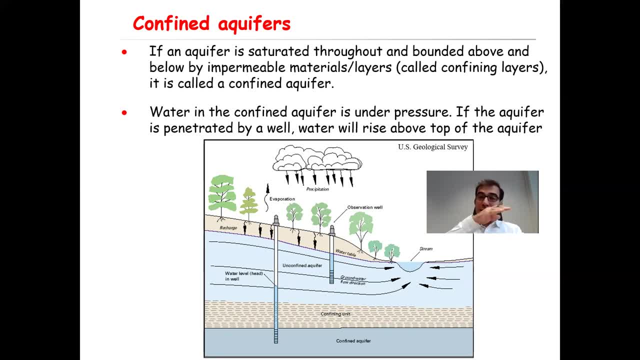 So it's a confined aquifer. So it's a confined aquifer. If an aquifer is saturated and from below and above it is bounded by impermeable layer, OK, by impermeable geological formations, that is a confined aquifer. 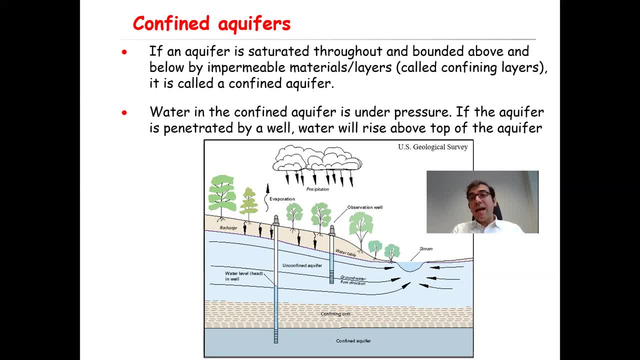 So if an aquifer is saturated throughout and bounded above and below by impermeable materials, layers called confining layers, it is called a confined aquifer. So look at this example, This water here you see from the top. it is confined by this impermeable layer. 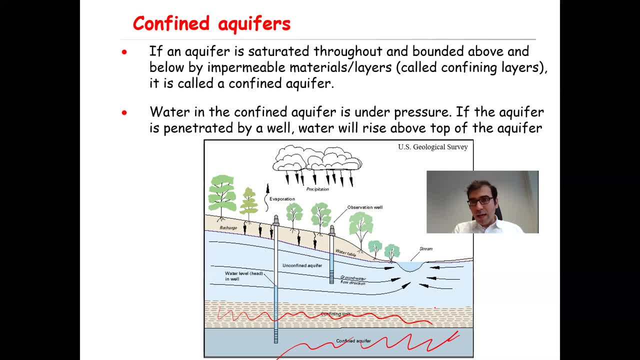 This water. here you see from the top. it is confined by this impermeable layer, which is presented by the brown color. OK, impermeable geological formation, let's call it confining layer, and therefore this type of aquifer is called confined aquifer. 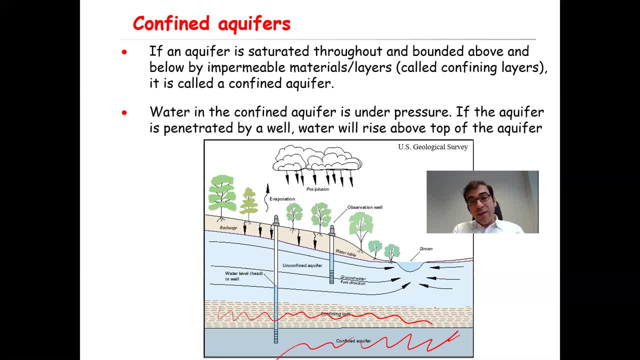 And notice that. note that the water in the confined aquifer is under positive pressure. In other words, if you penetrate this confined aquifer with a well, the water will rise above top of the aquifer. OK, So let me read. 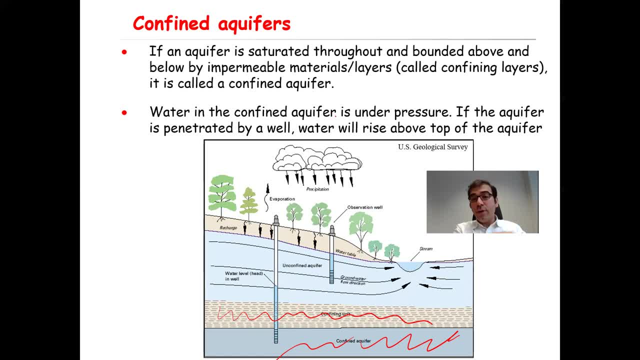 Let me read this from here. Water in the confined aquifer is under pressure. If the aquifer is penetrated by a well, water will rise above top of the aquifer, So that is confined aquifer. Another type of aquifer is called unconfined aquifer. OK, 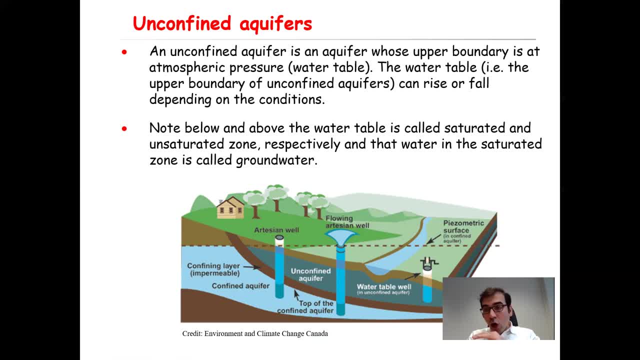 An unconfined aquifer at the top. at the top of the unconfined aquifer there is not impermeable formation. Basically, what that is is that the pressure is at atmospheric pressure And there is water table at the top of the unconfined aquifer. 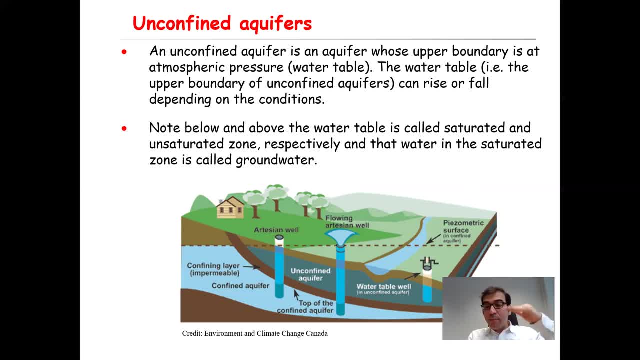 And water table is the kind of an interface separating the saturated zone- that is, anything below the water table is completely saturated- from the unsaturated zone. That is the thing. the region that is located above the water table- OK, So an unconfined aquifer- is an aquifer whose upper boundary is at atmospheric pressure water table. 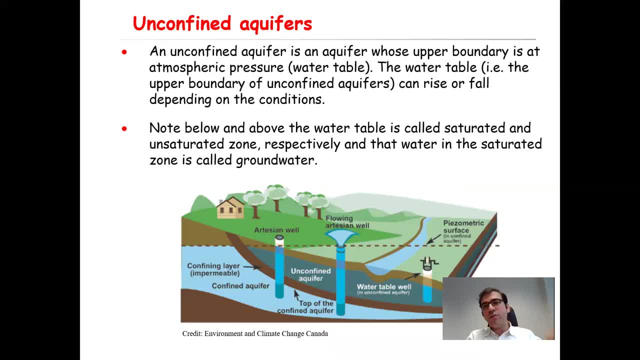 The water table that is the upper boundary of the unconfined aquifer, And where water table is located versus the unconfined aquifer is the direction in which the unconfined aquifer can rise or fall depending on the conditions. OK, 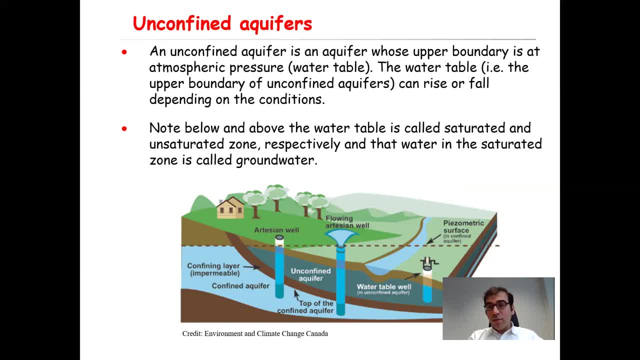 Note: below and above the water table is called saturated and unsaturated zone respectively, as I already explained, And that water in the saturated zone is called groundwater. So here in this cartoon you see this light blue in here. this is confined aquifer. 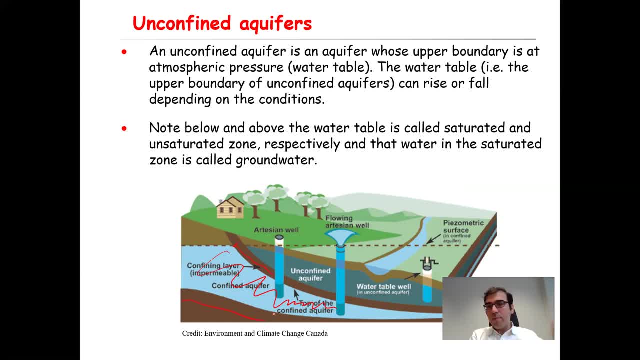 Because from the top and bottom, it is confined by impermeable layers presented by the brown color. But this aquifer, here, this one is, This is a confined aquifer, is an unconfined aquifer because at the top, there is no impermeable layer and at the top of the 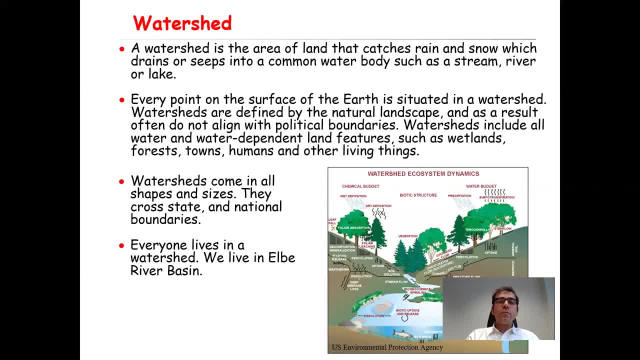 unconfined aquifer, there is water table. Another definition is watershed, which is another term that is used quite often in hydrology. What is a watershed? Basically, a watershed is the area of land that catches rain and the snow which drains or seeps into a common water body, such as a stream. 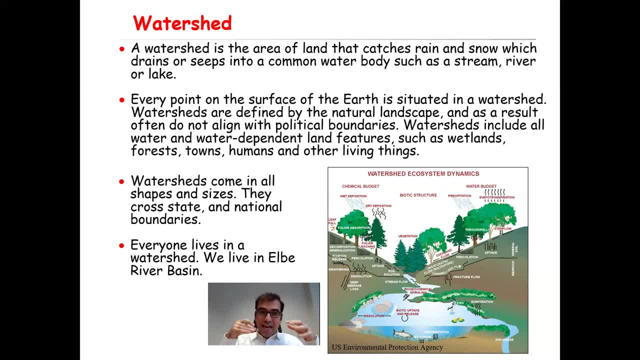 river or lake. So the area that collects the water and drains or seeps into the same water body is called a watershed and this cartoon shows a kind of a schematically, a kind of a typical watershed. Every point on the surface of the earth is situated in a watershed, Watersheds. 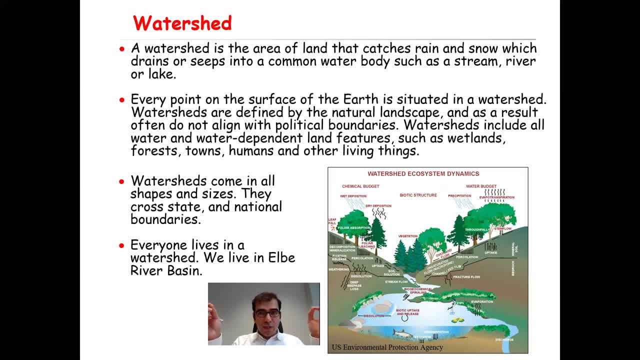 are defined by the natural landscape. Watersheds are defined by the landscape. Othersheds can be defined by the landscape, as hills, for example, and, as a result, often don't align with political boundaries, Which is what I like about watersheds, so that it can easily cross their political boundaries, because they 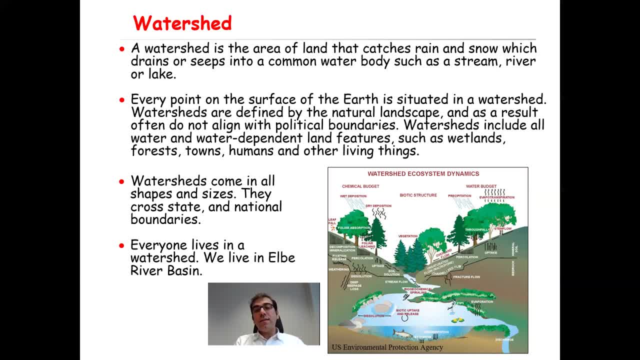 are not defined by the political boundaries but by the landscape. Watersheds include all water and water dependent land features such as wetlands, forests, towns, humans and other living things. okay, So watersheds come in all shapes and sizes. Sometimes they are very small and sometimes they can easily cross the border. 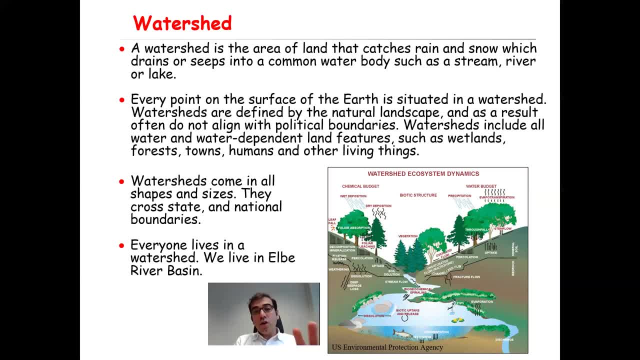 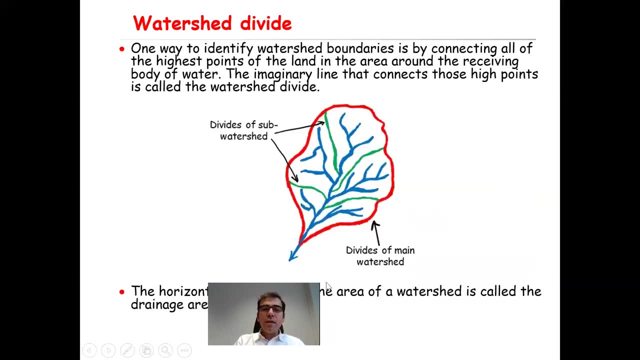 cross the states, across the countries and so on. so watersheds come in all shapes and sizes. they cross the state and national boundaries and everyone lives in a watershed. we living in Hamburg live in in Elbe river basin. okay, so that's the definition of watershed. another term is called 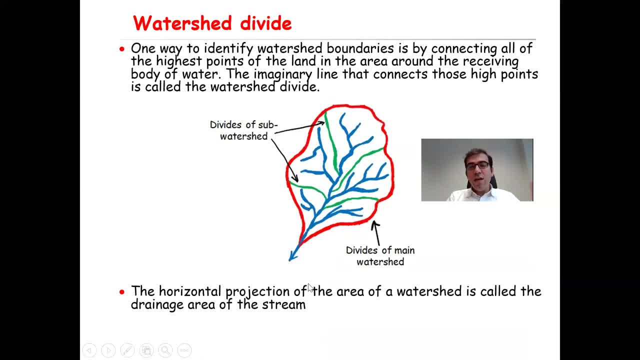 watershed divide. basically, that's the boundary of the watershed. okay, one way to identify watershed boundaries is by connecting all of the highest point of the land in the area around the, in the area around the receiving body of water, the. basically, if you connect these high points, the imaginary line that connects those high points points is called the watershed divide. so in this, 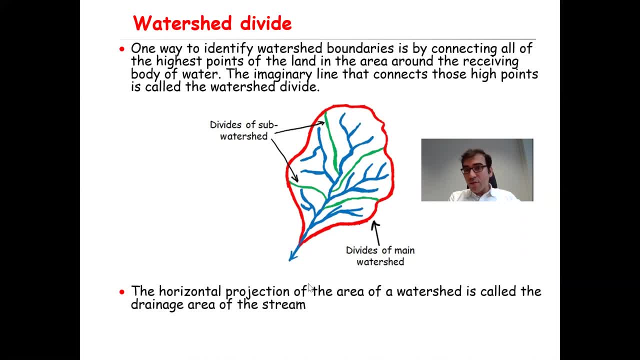 picture you see here. this red boundary is the divides of the main watershed and these green boundaries are the divides of the sub watersheds. okay, and the horizontal projection of the area of a watershed is the division of the main watershed and the horizontal projection of the 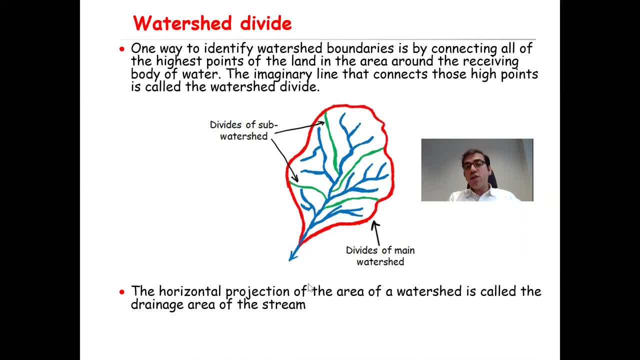 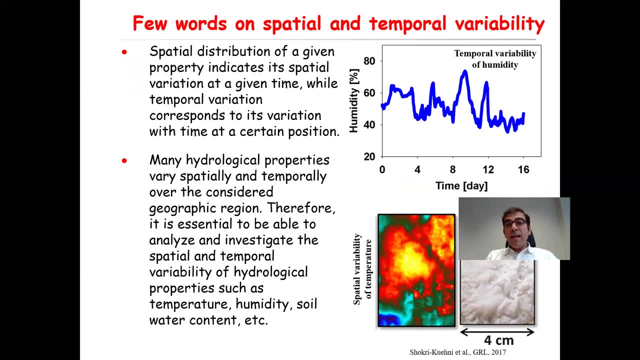 watershed- this is another definition- is called the drainage area of the stream. so the horizontal projection of the area of a watershed is called the drainage area of the stream. okay, and now a few words about a special and temporal variability. a special variability of a given property indicates a special variation at a given time. okay, so for a certain time you wanted to see. 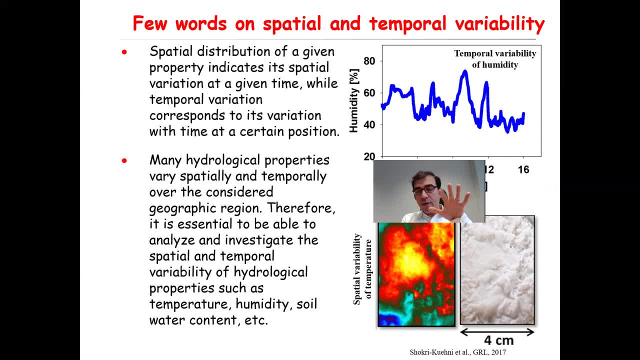 how a particular quantity, let's say temperature for example, varies across the space, that is called a special variability, while temporal variation corresponds to its variation, the variation of that quantity with time at a certain position. for example. look at this figure at top: this is humidity versus time at a certain spot. so at a certain spot i'm measuring, let's say, with the 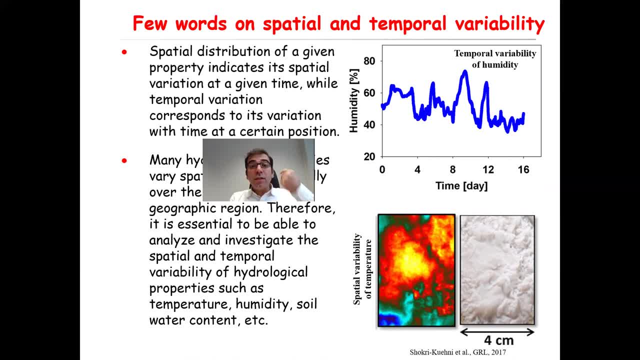 sensor, the how humidity changes over time. so that is called temporal variation, okay, or temporal variability, and, on the other hand, a special variability. for the special variability, look at the picture at the bottom. so here this is actually one of our research results that is probably that was published in geophysical research letters in 2017, where we looked into the temperature value. 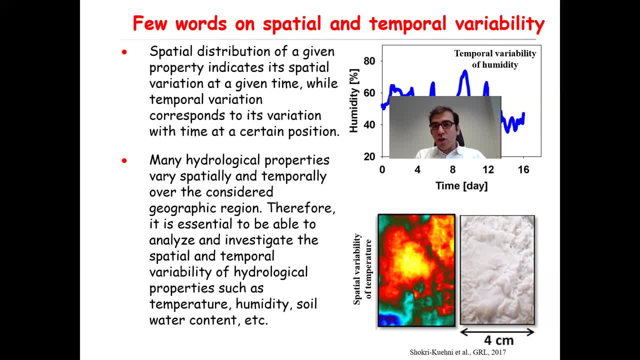 temperature variation at the surface of the cross, salt cross formed as a result of evaporation. okay, so here on the right side, the white color here is the precipitated salt or crystalline salt on the surface of sand on the drawing. okay, and on the left it's the thermal picture showing. 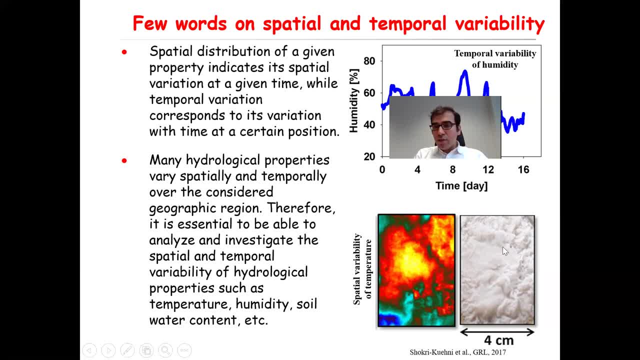 the temperature distribution across this, throughout this salt cross, basically okay. so in other words, let's say, after i don't know- 10 hours or 15 hours from the onset of the experiment, we take a thermal picture at a certain time and at that time we are looking to the variation of the temperature across. 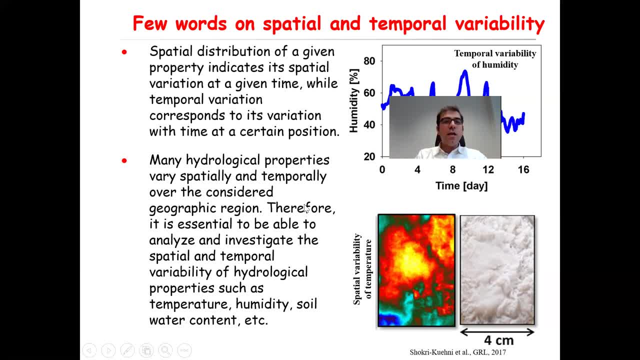 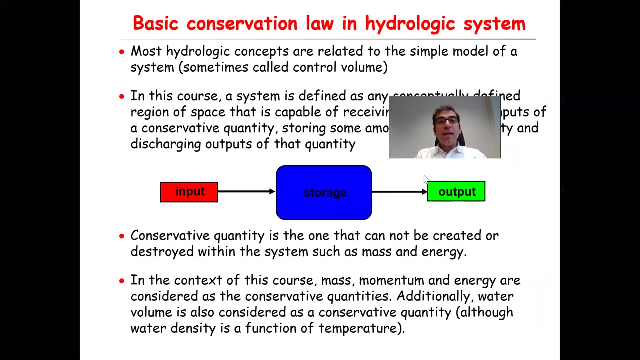 the space, and that is called a special variability. okay, so many hydrological properties vary, especially temporally, over the considered geographic region. therefore, it is essential to be able to analyze and investigate the special and temporal variability of hydrological properties, such as temperature, humidity, salt water content, etc. okay, and now let's talk a little bit about. 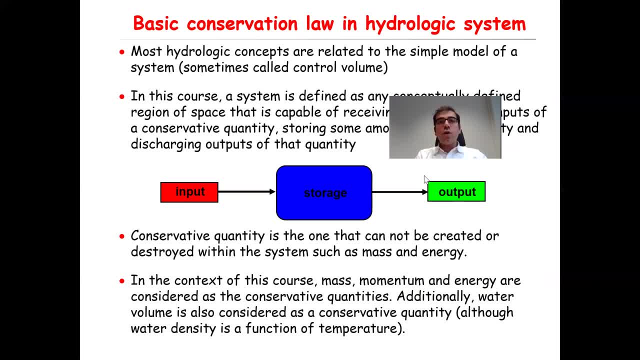 basic conservation law in hydrologic system. so most hydrologic concepts are related to the simple model of a system and or sometimes called control volume. in this case, we are talking about the system of the system, of the system, of the system, or sometimes called control volume. in this, 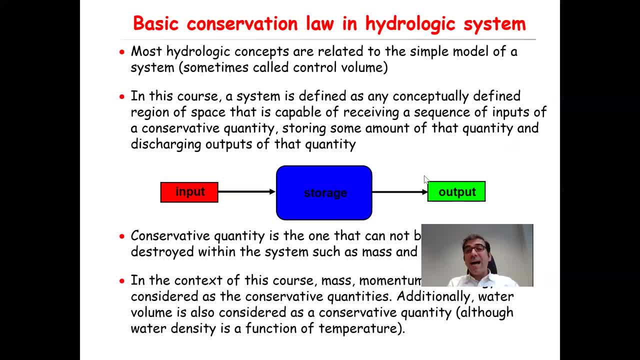 course a system. what is a system? a system is defined as any conceptually defined region of a space. okay, that is capable of receiving a sequence of inputs of a conservative quantity, storing some amount of that quantity and then discharging outputs of that quantity. so here you see, here. 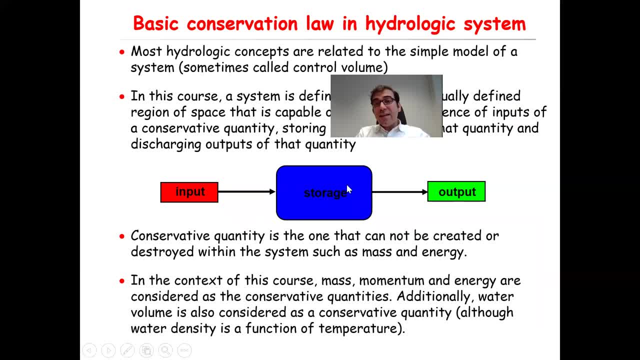 you have the input. some part of that is stored here and another part is discharged in terms of as as output. okay, that is for us a system. okay, and and what is conservative quantity? by the way, conservative quantity is the one that cannot be created or destroyed within the system, such as mass and energy, and in the context of 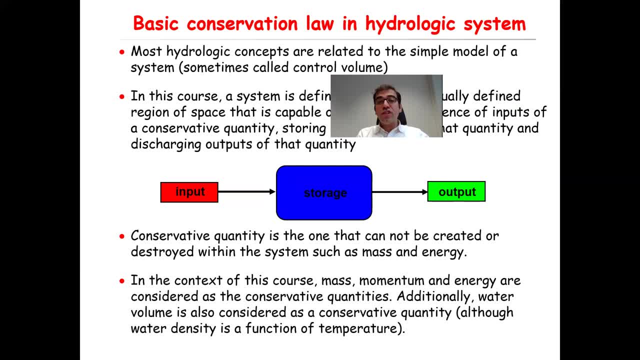 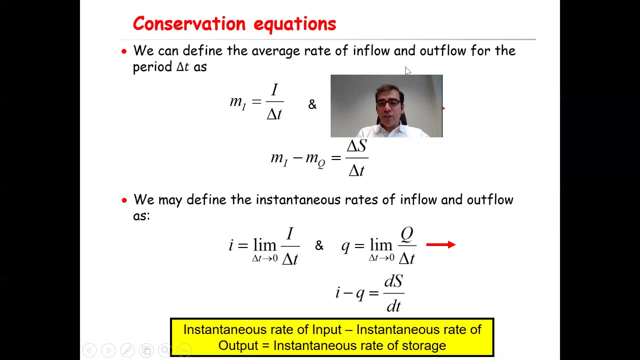 this course, mass momentum and energy are considered as the conservative quantities. additionally, water volume is also considered as a conservative quantity, although water density slightly changes as a function of temperature. but in this course we assume water volume is a conservative quantity. okay, so you can express that previous explanation. 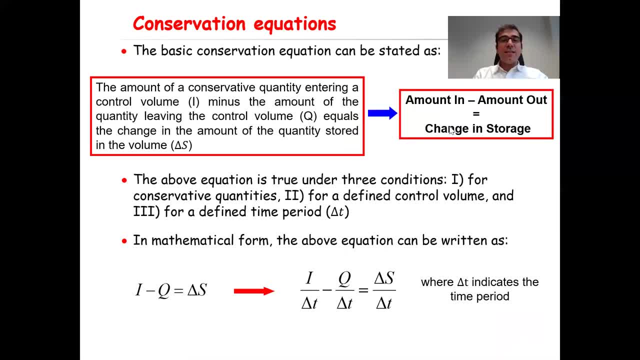 in. in mathematical form: uh, that is basically the basic conservation equation can be stated as: the amount of a conservative quantity and, entering the control volume- let's present it by i, minus the amount of the quantity. leaving the control volume- let's present it by q- equals the change in the 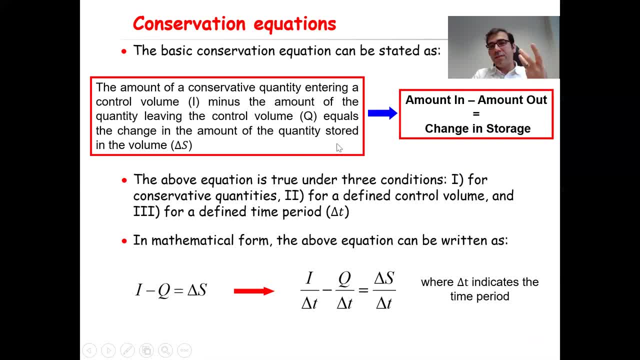 amount of the quantity as stored in the control volume, that is delta s. basically, it says amount in minus, amount out is equal to change in the storage. but remember, you must meet three criteria to be able to apply this equation. that is very important. the first one, the above equation, is true under three conditions. the first one is for conservative. 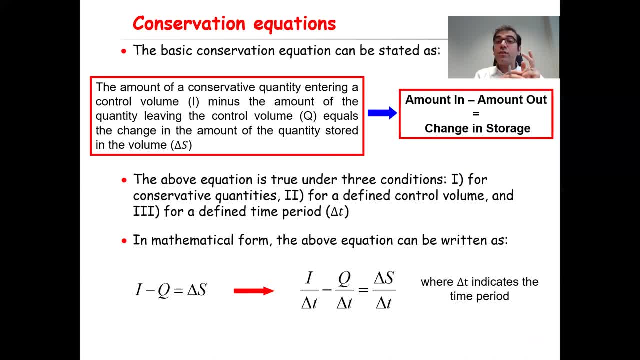 quantities, so the quantity should be conservative. the second one is for a defined control volume and the third one is for a defined time period. delta t. okay, so in the mathematical form you can write amount in as i minus m out, as q is equal to delta s. that is the change in the 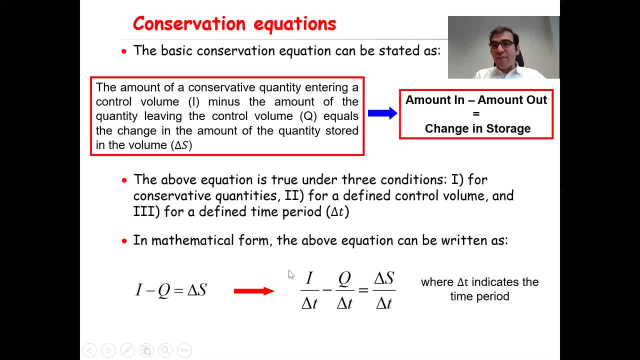 amount of the quantity stored, or you can write it as a kind of average quantity. okay, over that period of time that you can divide everything by delta t, that will be i divided by delta t minus q. divided by delta t is equal to delta s divided by delta t. and delta t indicates the time period. okay, so 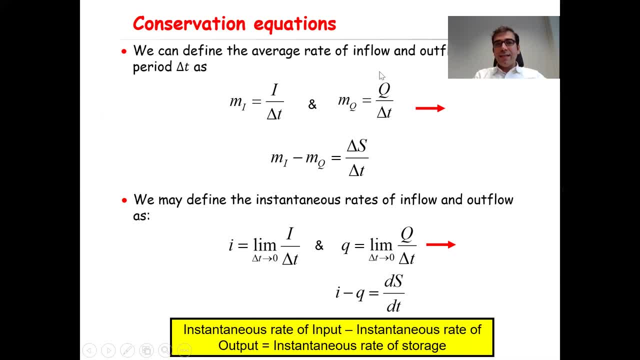 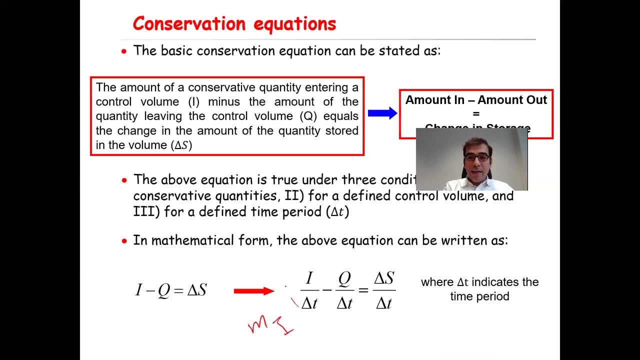 if you present i divided by delta t as the average rate of inflow by m i, the term m, i and q divided by delta t by m q, so you can write the previous equation, remember i divided by delta t. you can write m, i and q divided by delta t. you. 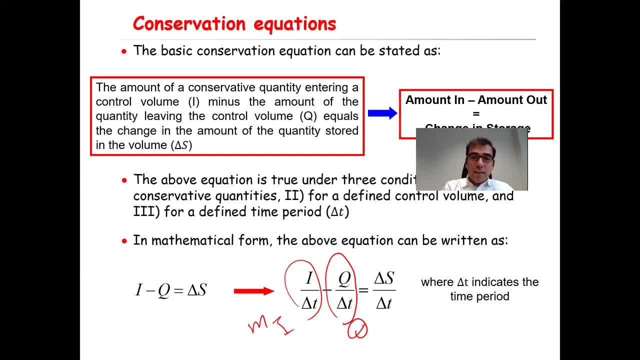 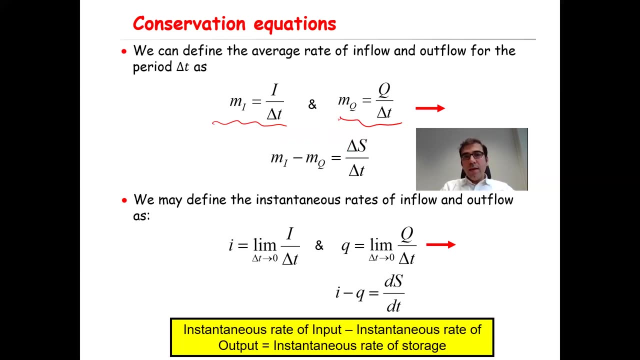 can write m q. you can write it as: uh, sorry, you can write it as m q, so i m i minus m q. m i minus m q is equal to delta s over delta t. okay, uh, that is the average rate you can as well consider. you may want to define the instantaneous rates of influence. 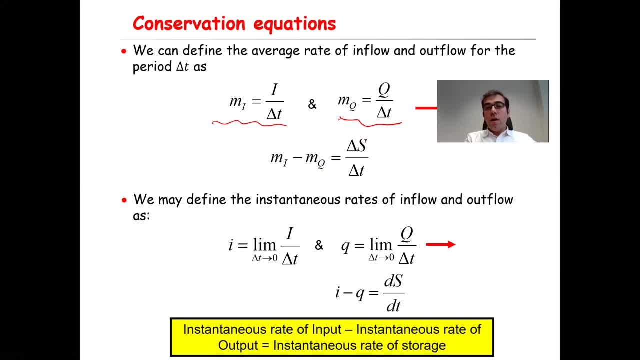 outflow and for that you need to take the derivative of uh i. basically, with respect to uh t, that is limit i divided by delta t when delta t go 10 to 0, or q, that is limit q divided by delta t when q delta t tends to 0. that means i minus q is equal to derivative of s. with respect. 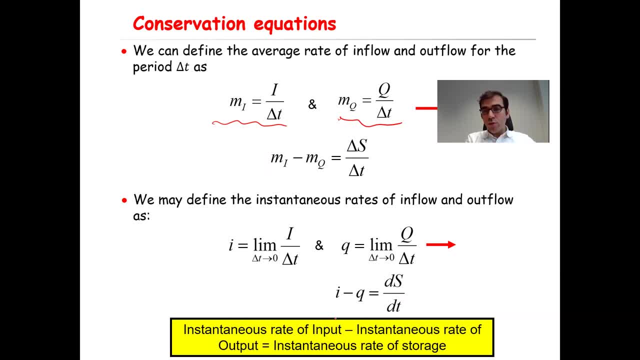 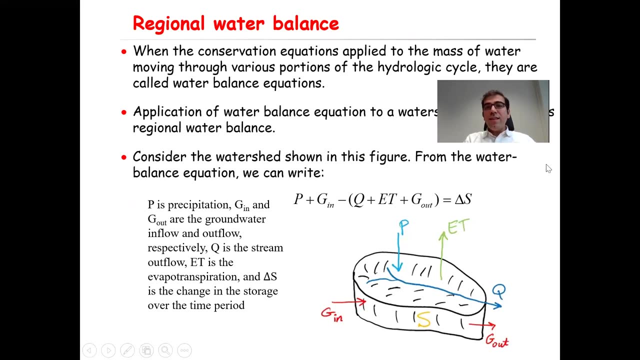 to t. okay, that is instantaneous rate of our input. little i uh minus instantaneous rate of output. q is equal to instantaneous rate of storage. okay, so that is the conservation conservation equation. so what is regional water balance? so when the conservation equations is applied to the mass of 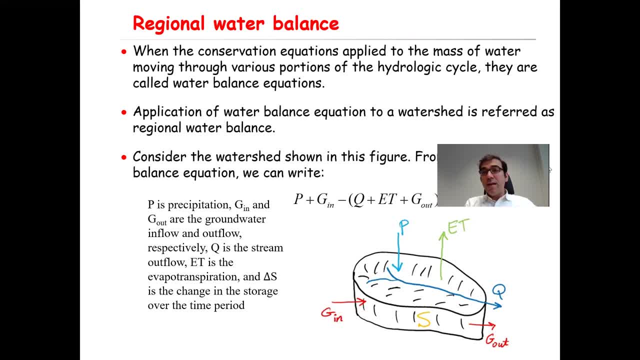 water moving through various portion of the hydrologic cycle. they are called water balance equation. so basically, when you apply the conservative conservation equation to muscle water moving in the environment moving through the hydrologic cycle, that is called water balance equation. and then when you apply the water balance equation, 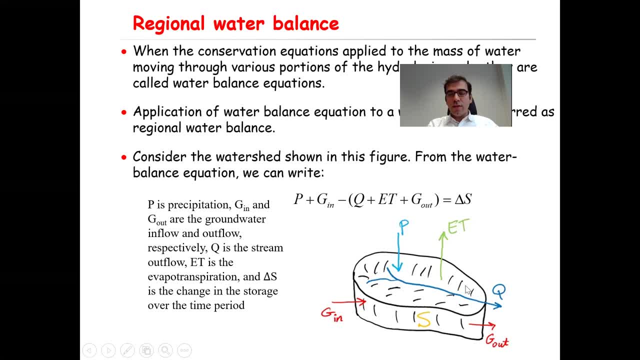 actually write it down in a mathematical form. let's consider this, this water watershed. okay, so again the same story. input minus output is equal to delta s. what is the input here? in a watershed, the. in water, the the input is p, that is precipitation, plus g in, that is ground for. 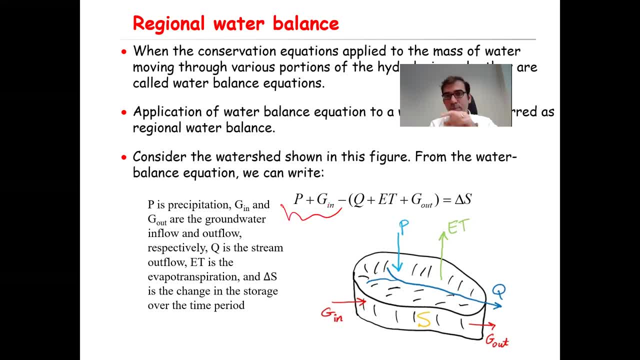 groundwater inflow. that is. so these two terms is ei, the input minus the output, that is evapotranspiration. et, that is the q stream outflow and that is the groundwater outflow. so q plus et plus g out, that is the i minus q, is equal to delta s. so that is basically the regional water balance. okay. 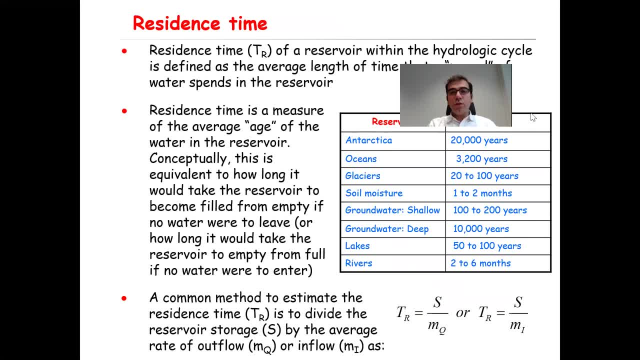 and so another term that i like to introduce here is the residence term that is as well quite often used in in hydrologic analysis: the residence, sorry residence time. so residence time that is quite often used in hydrologic analysis and residence time is presented by tr: our residence time of the 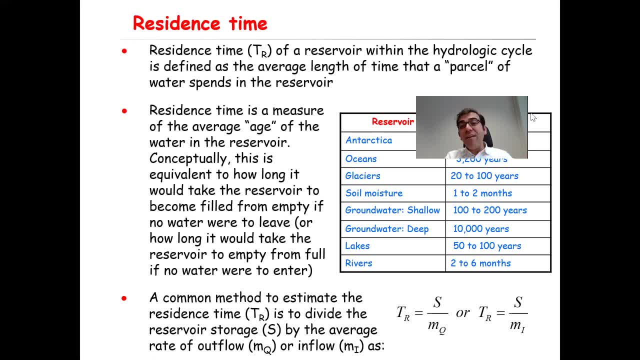 reservoir within the hydrologic cycle is defined as the average length of time: average length of time that a parcel of water spends in the reservoir. okay, you can either consider that the kind of residence time is a measure of the average age of the water in the reservoir. okay, 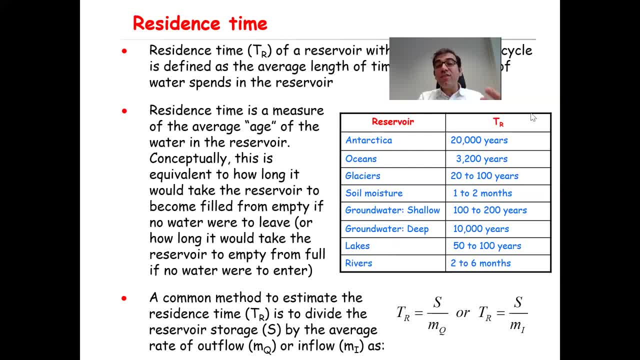 and conceptually this is equivalent to how long it will take the reservoir to become filled for from empty if no water were to leave. or you can as well say how long it would take the reservoir to empty from full if no water were to enter. okay, and this table provides some typical values, some 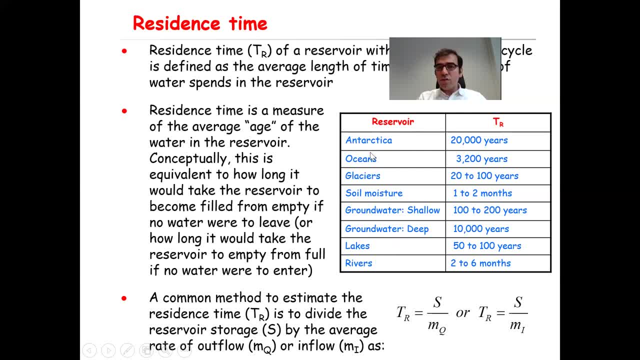 average values of the residence time of different reservoirs. you see, i see here antarctica 20 000 years, oceans 3 200 years, and i don't know. groundwater, when it is shallow 100, 200 years, when it is deep ten thousand years, river two to six months and soil moisture one to two. to three months. quite short, actually. so this is the typical value for the res for the residence time of different reservoirs, and a common method to estimate the residence time, tr, is to divide this reservoir storage s by the average rate of outflow s divided by mq. okay, that will be tr, or. 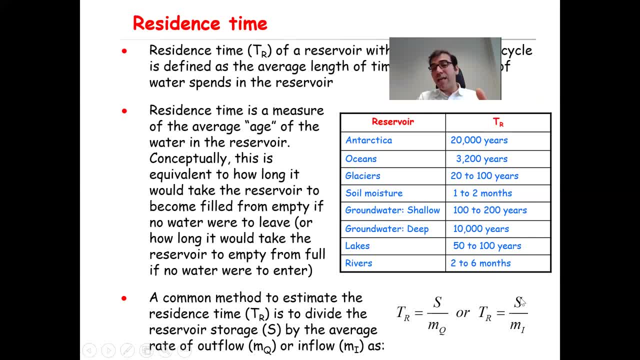 you can as well divide s that storage by the average rate of inflow, mi, so s divided by m divided by mi or s divided by mq. it's a common method to estimate the residence time, okay, so here i'm going to say a few words about dimensions. 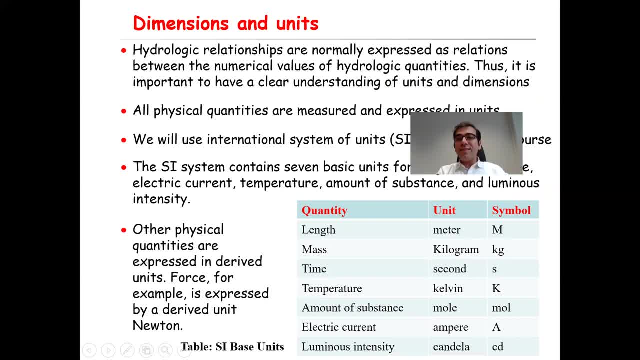 and units. so, as you know, units is the quantitative expression of a quantity, but dimension is the qualitative expression of the quantity, in other words, actually let me go through this one. so hydrologic relationships are normally expressed as relations between the numerical values of hydrologic quantities above a minimum or unit. but you see the data already. would not be a question. okay, it's. 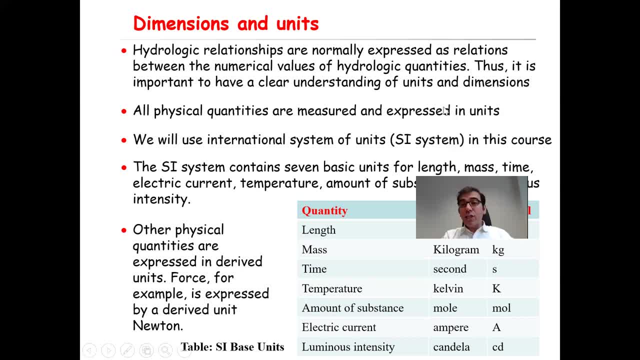 a very important to have a clear understanding of units and dimensions. all physical quantities are measured and expressed in units. okay, we will use international system of units, that is, SI system, in discourse. the SI system contains seven basic units. okay, for length, mass time and so on. all of 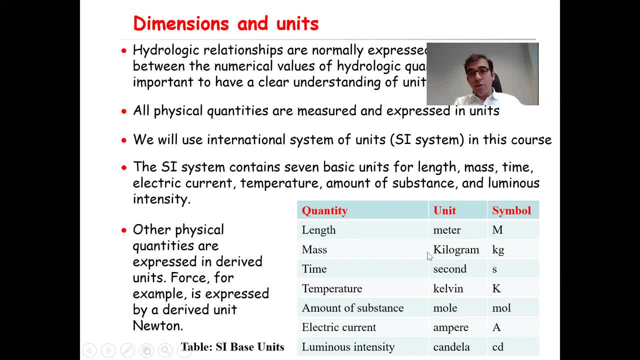 And these are the SI units: for length is meter, for mass is kilogram, for time is second, for temperature is Kelvin, and so on. And these are the symbols that are used to present these units. So other physical quantities are expressed in derived units. 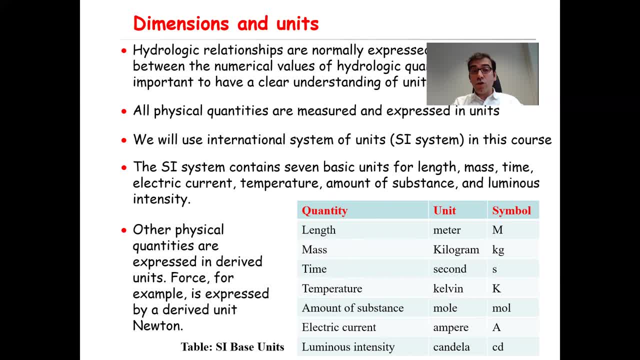 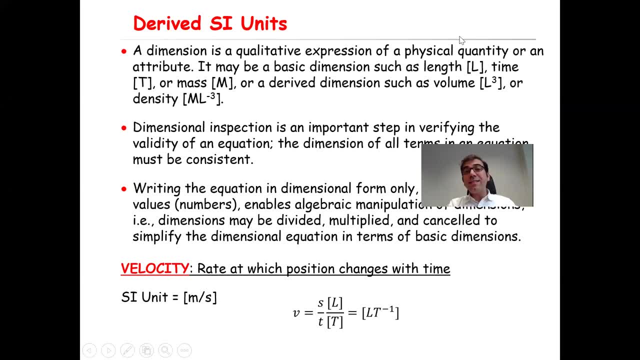 Force, for example, is expressed by a derived unit that is called Newton. OK, so dimension, as already mentioned, is a qualitative expression of that physical quantity or an attribute. It may be a basic dimension, such as length, OK, time. 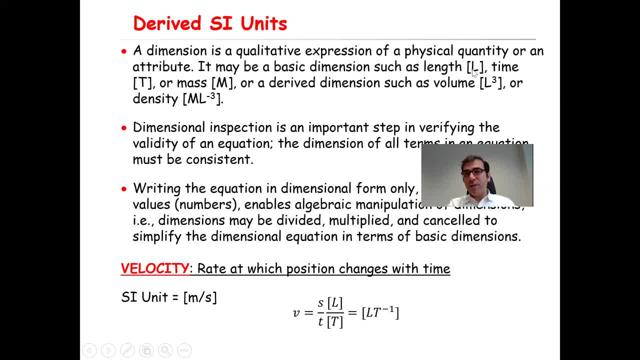 So it may be a basic dimension, such as length presented by L, time presented by T, or mass presented by M, or a derived dimension such as volume, That is, L, L with the power of T, L cubic, or density, M divided by L3.. 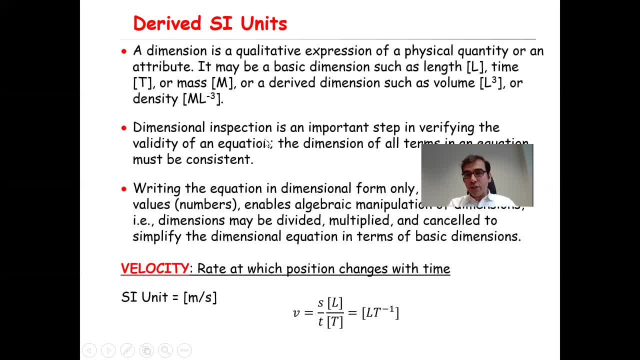 OK, so that's dimension. So dimensional inspection is a powerful tool to verify the validity of an equation. You know the word. dimensional inspection is an important step in verifying the validity of an equation. The dimension of all terms in an equation must be consistent. 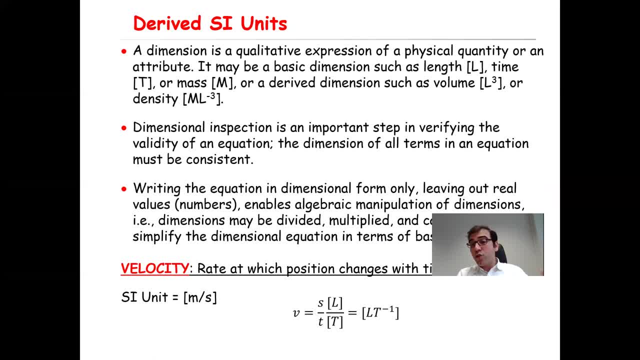 So if the dimensions are not consistent, that means something is wrong with that equation. OK, and Writing the equation in dimensional form only, leaving out real values, numbers, enables algebraic manipulation of dimensions, that is, dimensions may be divided, multiplied and cancelled to simplify the dimensional equation in terms of basic dimensions. OK. 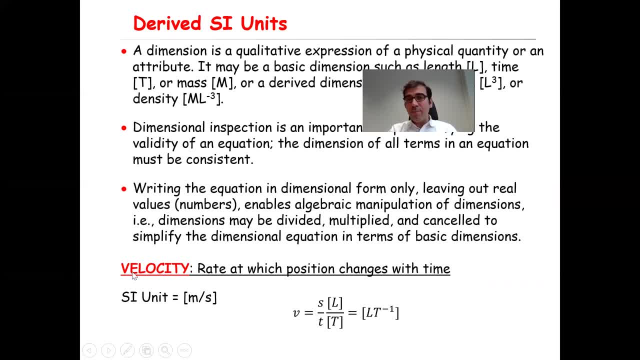 So velocity. so let's actually solve a couple of examples. I wanted to show you how to derive the dimension of a given quantity, So velocity. velocity is rate at which position changes with time. right, So it is calculated by V. velocity is equal to S divided by T and S. the dimension of S is L and the dimension of T is the capital T. therefore, the dimension of the velocity is LT minus one, and the SI unit of velocity, as you may know, is a meter per second. 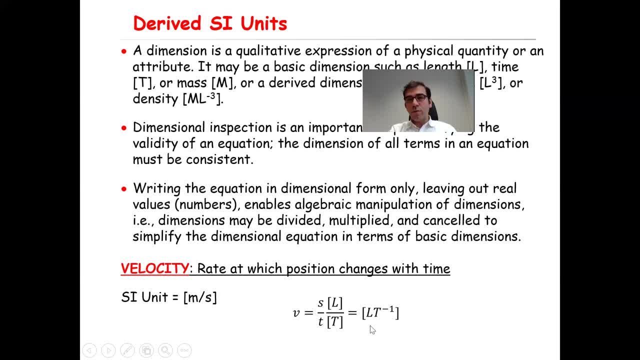 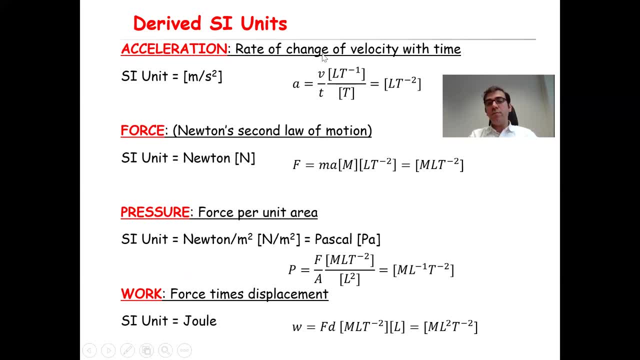 So that's the dimension of the velocity LT minus one. So you can do the same calculation, for example, for acceleration, that is, rate of change of velocity with time. The SI unit is meter per square second. Acceleration is equal to velocity divided by T. 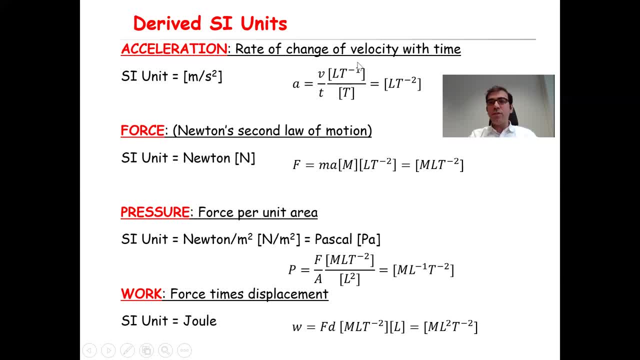 Velocity is LT minus one, the dimension. We calculated the previous slide divided by T, which will be LT minus two. Another one is force. That is Newton's second law of motion. The SI unit of force is Newton and F is equal to M? A. 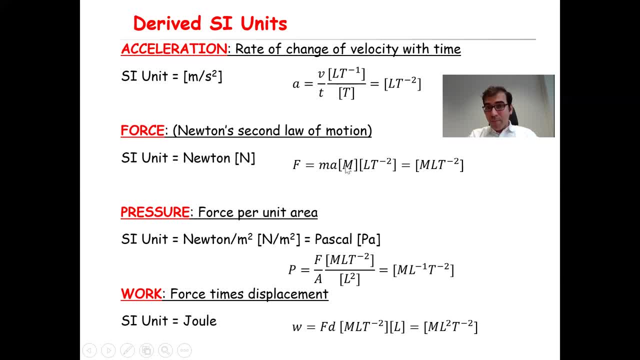 M is the mass. the dimension of M is M. based mass is M. the dimension of acceleration is LT minus one. The S is equal to N. The S is equal to T minus two. The S is equal to T minus three. 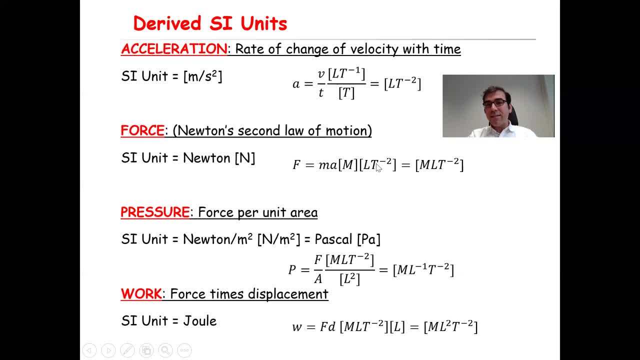 The SI unit isccel t. Therefore the dimension of force will be mLt minus 2.. That's mLt minus 2.. Pressure, that is force per unit area. The SI unit is newton per square meter, or represented by n divided by m square, or it is called as well Pascal, presented by PA. 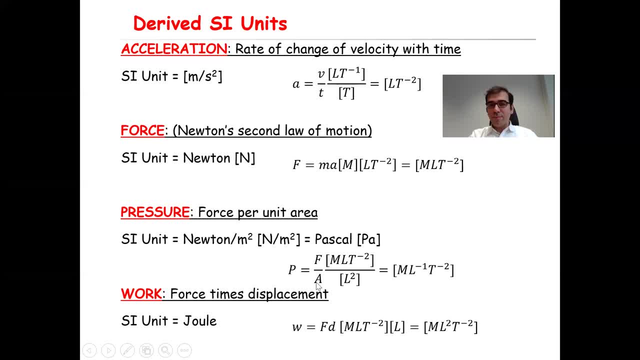 And in terms of dimension, P pressure is equal to F. divided by A, F is mLt minus 2.. So we have it here, That is mLt minus 2.. You just plug it here. Divided by A, that is L square. Therefore, this one will be mL minus 1, T minus 2.. That will be the dimension of pressure. 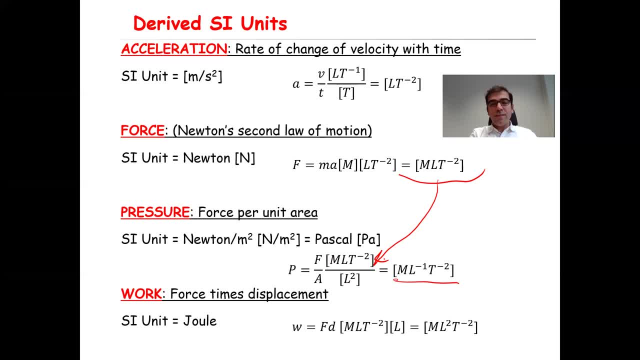 And dimension of work is for the definition of work. basically is force times displacement? Okay, the SI unit is joule And the equation is: work is F, F is force, The dimension of force. we just calculate. sorry, not this one, We just calculated the dimension of the force. You plug it here. That is mLt minus 2 times dimension of D is L, That will be mL2 T minus 2.. 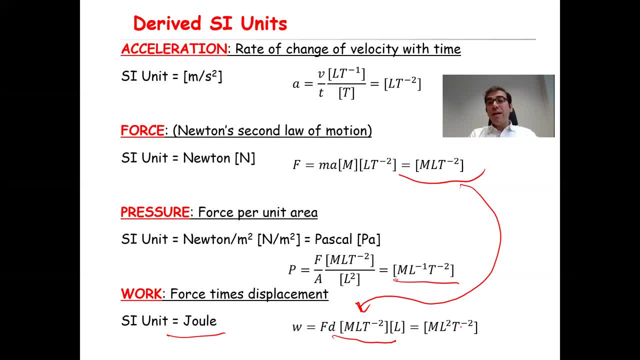 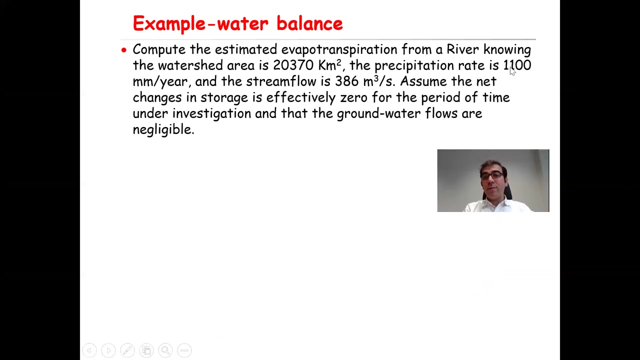 So there were a couple of examples on how to calculate the dimensions of other quantities using the dimension of those seven quantity mentioned, Okay, Basically in this table. Okay, Okay, so I have now one example and then that will then conclude this lecture. So the example is about water balance. Okay, so the question is: compute the estimated evapotranspiration from a river, knowing the watershed area is 20,370 square kilometer. 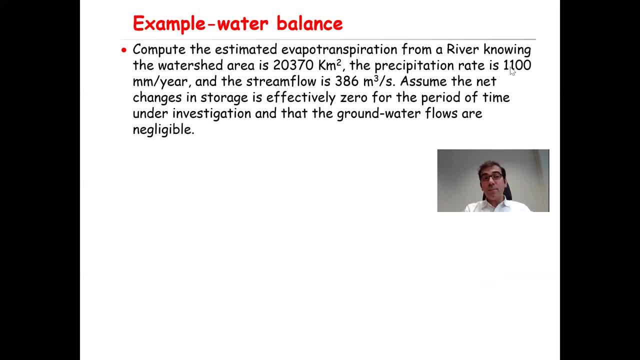 The precipitation rate is 1,100 millimeter per year and the stream flow is 370.. Okay, And thus the data can be selected as follows. The temperature of the river is 286 cubic meters per second. Assume the net changes in the storage is effectively zero. That means delta S is effectively zero for the period of time of the investigation and that the groundwater flows are negligible. That means G in and G out is equal to zero. Okay. 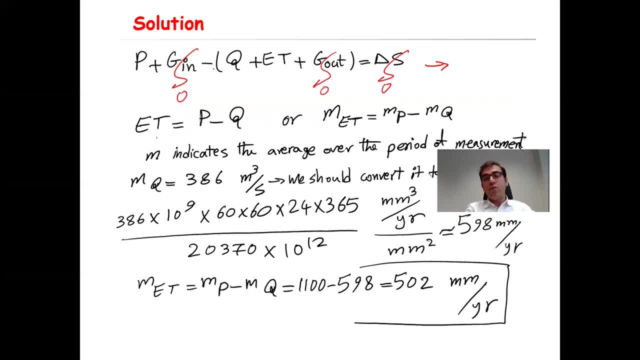 So basically to solve this question, you simply need to write the water, the regional water balancing equation, That is, P precipitation plus G in, minus Q plus ET plus G out is equal to zero, And that is what the data is. Okay. 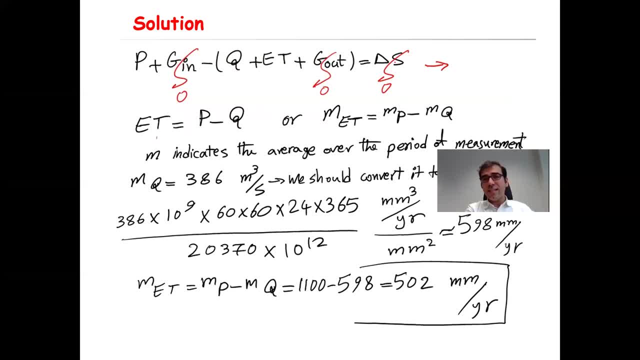 out is equal to delta s. The question itself says delta s is equal to zero. ignore the ground water flow. that is g in and g out is zero. so you can simply bring et to the other side of the equation. so therefore, et will be equal to p minus q Or, in the average term, average over time. you can write: 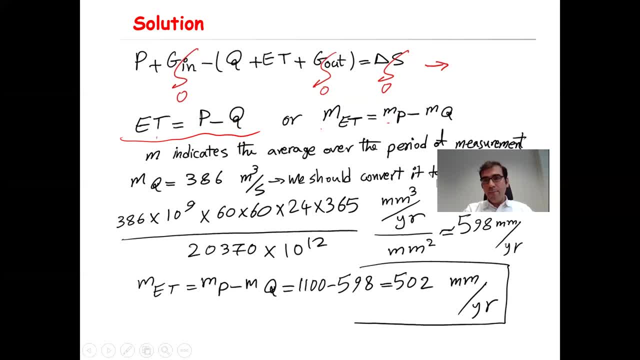 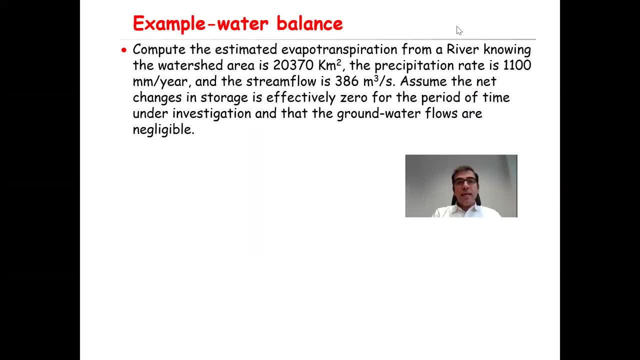 met equal to mp minus mq. okay, So in the question. so here, sorry, the precipitation rate is 1100 millimeter per year. okay, But the stream flow is in the unit of cubic meter per second, so we need to convert it to the unit of millimeter per year. okay, So that 386. 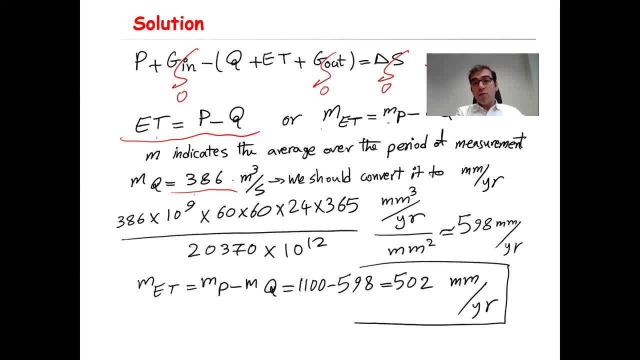 cubic meter per second. so remember, note that the precipitation is millimeter per year. so that is a kind of unit of velocity length per time. but this is volume per time. so you first need to divide this by the area to get the lengths per time. okay, But of course you need to convert. 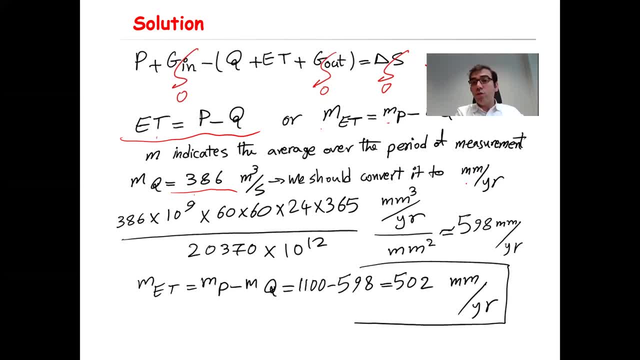 the units to be consistent. so here we wanted to work with the unit of millimeter per year. so we need to convert the units to be consistent. so here we wanted to work with the unit of millimeter per year. so cubic meter so 386, to convert cubic meter to cubic millimeter you need to multiply. 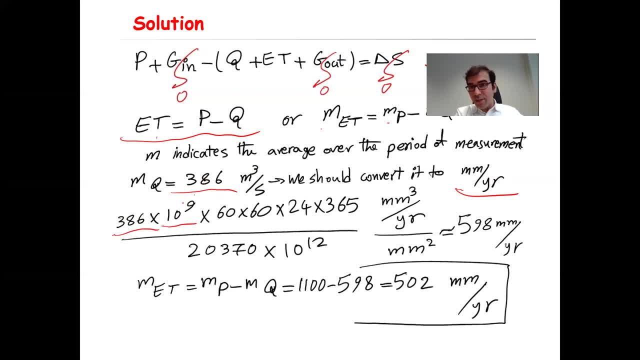 it by 10 to the power of 9, because 1 meter is 1000 millimeter, therefore a cubic meter will be. to convert it to cubic millimeter, you need to multiply it by 10 to the power of 9,.